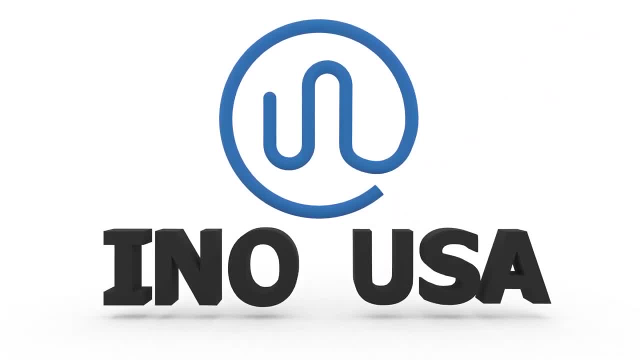 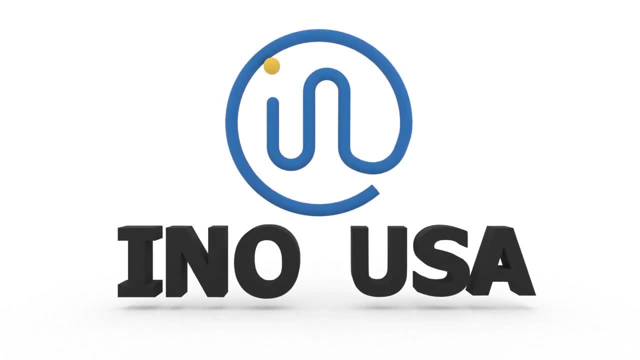 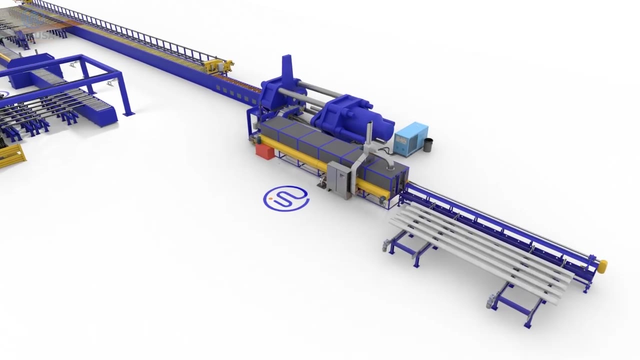 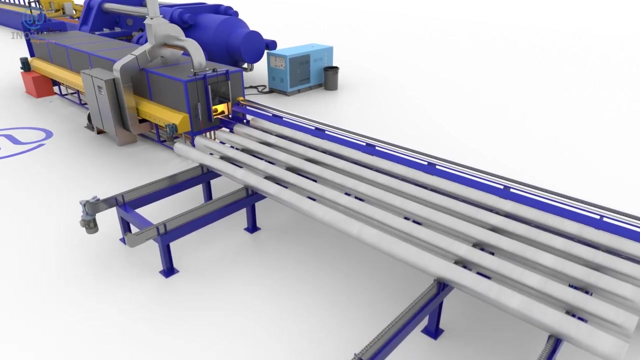 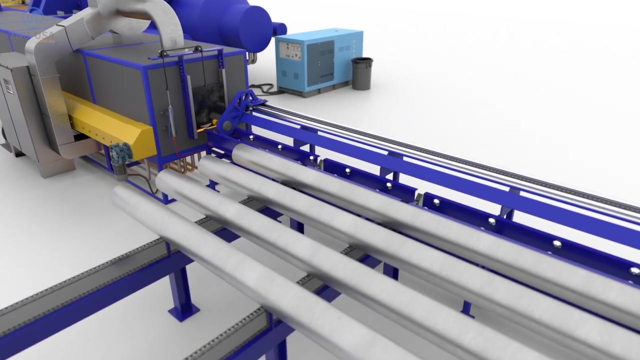 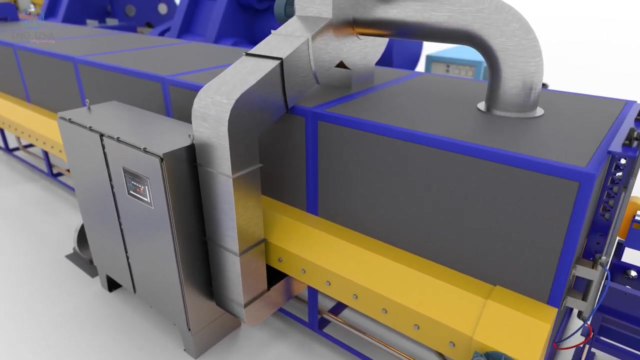 The aluminum extrusion process starts when an aluminum log or billet gets loaded on a furnace. The billet can have different diameters depending on the size of the profile we want to extrude In the furnace. it gets heated up to temperatures ranging from 600 to 1100. 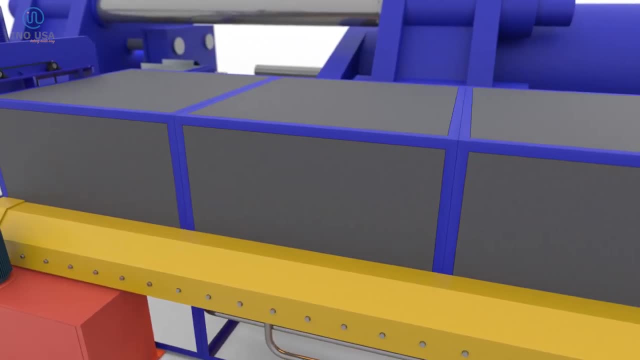 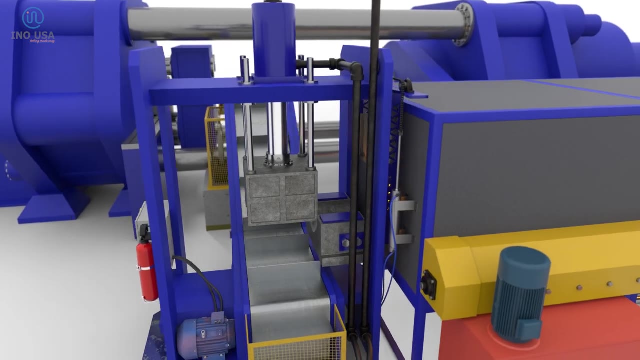 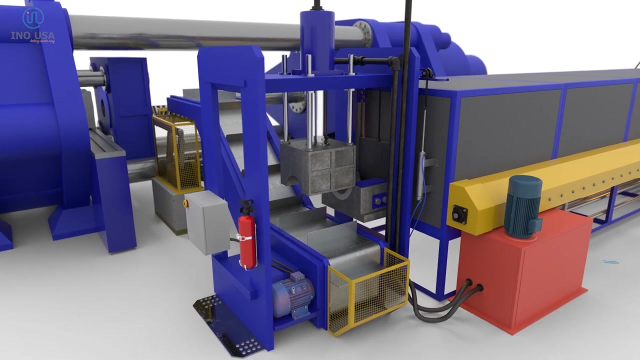 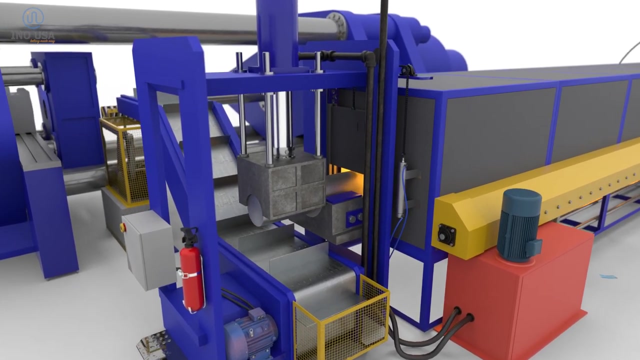 degrees Fahrenheit depending on the size of the log. Once the billet is soft enough it goes through a hot log saw that cuts a smaller size billet that will go through the extrusion press. The billet then gets transferred to the press via. 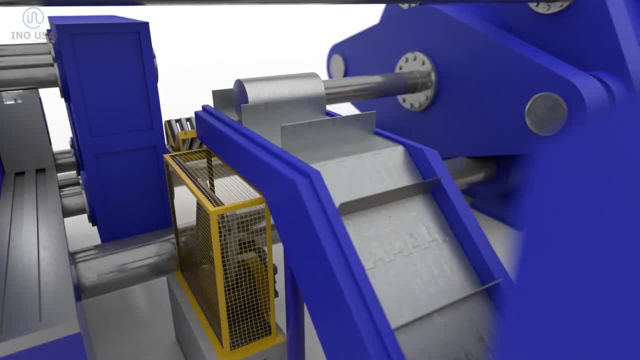 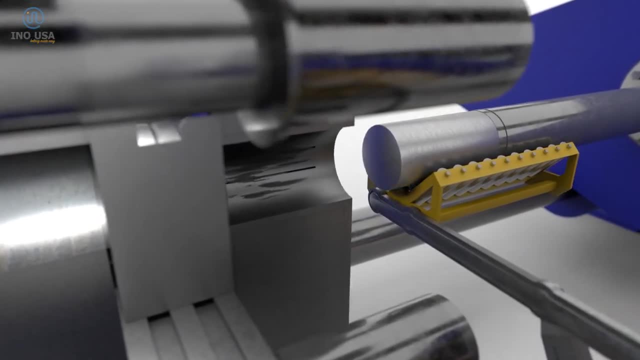 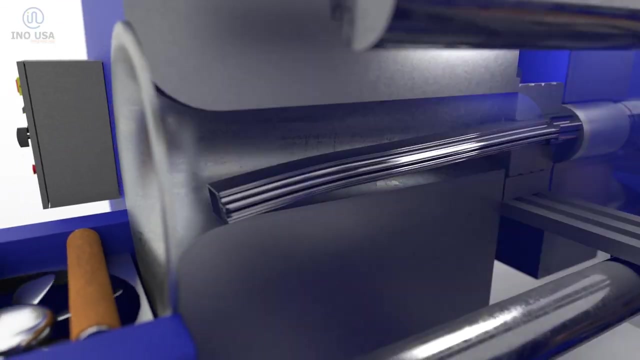 inclined metal conveyor belts or even automatic elevator systems. Once loaded, a hydraulic press pushes the soft aluminum through a die that will give it the desired shape. Presses can range from 1000 to 8000 metric tons. As the profile is extruded, it falls into what is called. 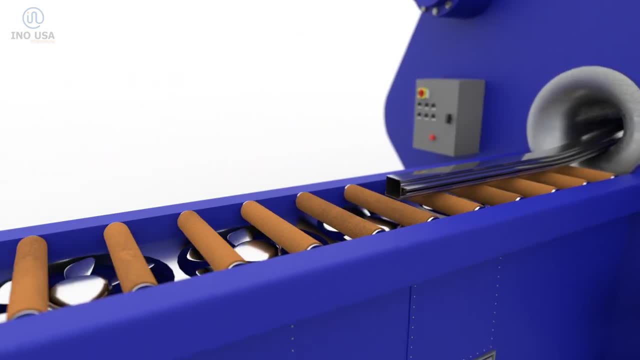 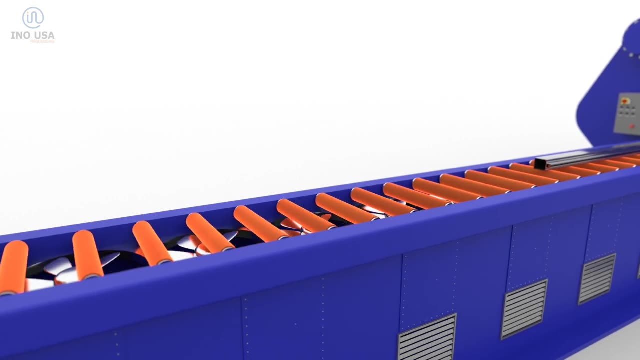 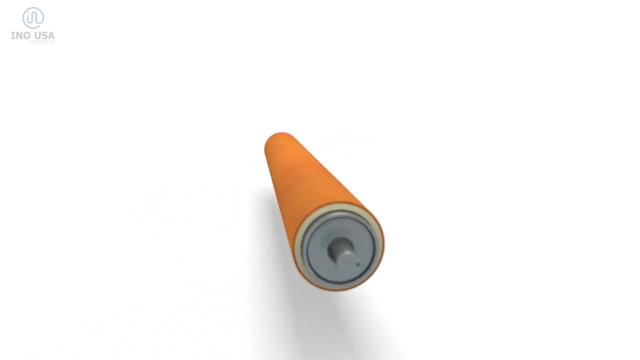 the lead-out table. Lead-out tables have metal rollers with felt covers that are heat resistant and non-marking. The roller covers featured on the lead-out table have to withstand the hottest temperature of the aluminum extrusion process. These are felt roller covers comprised of two. 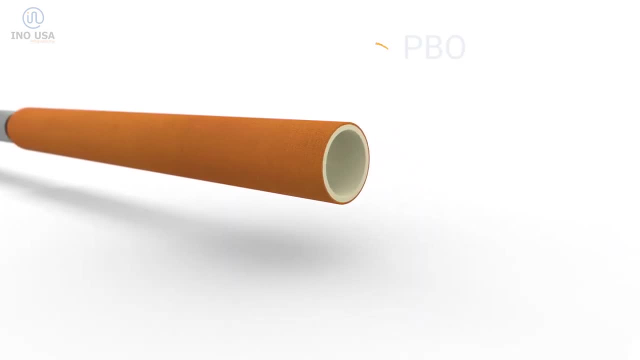 different fibers. On the top we have PBO. PBO stands for are you ready? Polybenzoxazole PBO is a synthetic fiber resistant to around 1200 degrees Fahrenheit for short periods of time. The bottom of the roller has aramid fibers, such as Kevlar, which is resistant to around 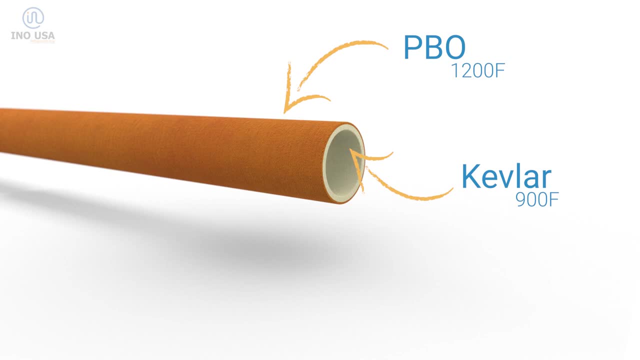 900 degrees Fahrenheit for short periods of time. This is done to lower the cost of the roller cover, Because PBO is a very expensive fiber. why waste that fiber on the bottom of the roller when the bottom is never ready? PBO is a synthetic fiber resistant to around 1200 degrees Fahrenheit for 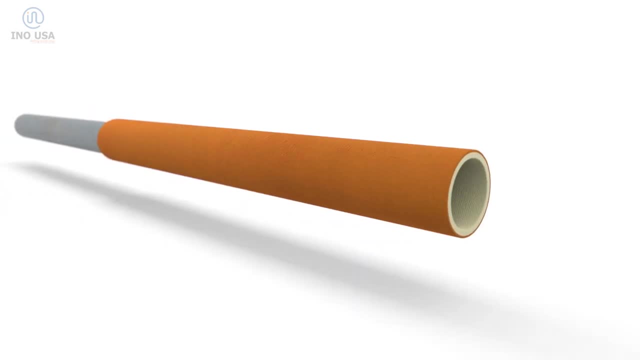 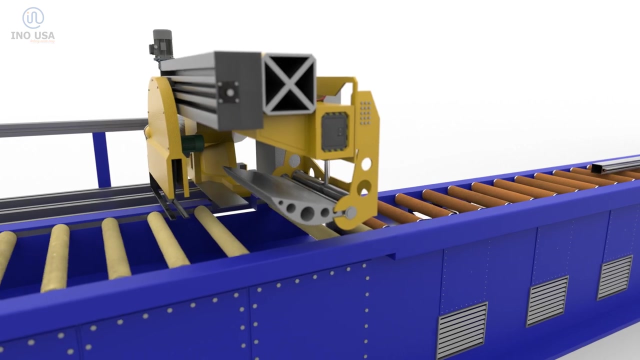 short periods of time. The amount of PBO versus Kevlar will depend on the size of the aluminum profile being extruded. The bigger the profile, the longer it will take to cool down and the more PBO fiber we need to use To help cool down the profile, faster the lead-out tables are equipped. 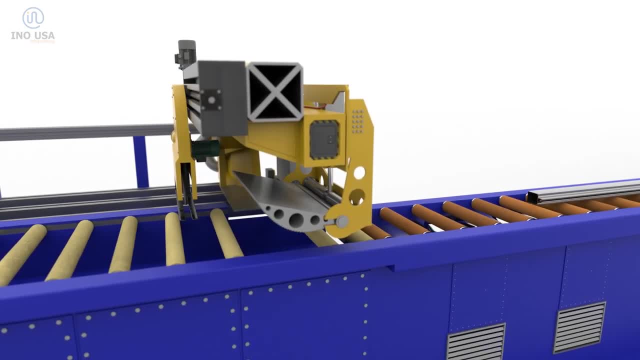 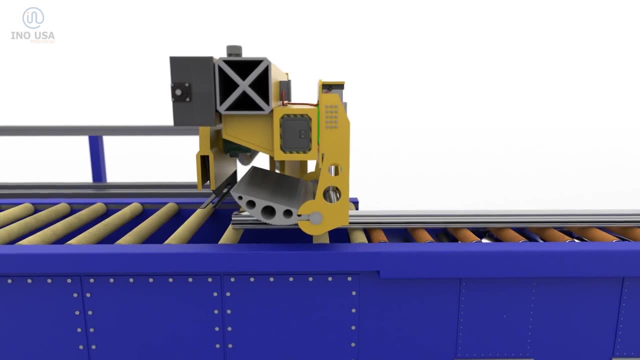 with cooling fans or ducts and sometimes even a flood quench that cools the profiles down by spraying water. A single head or dual head elevated puller, which is a very important element in a, helps pull the profile out of the press further down the line into what is called the run-out table. 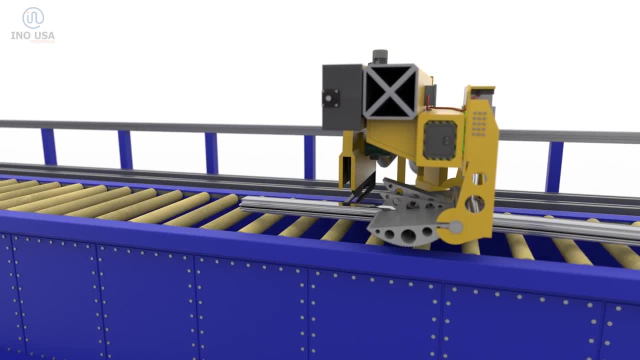 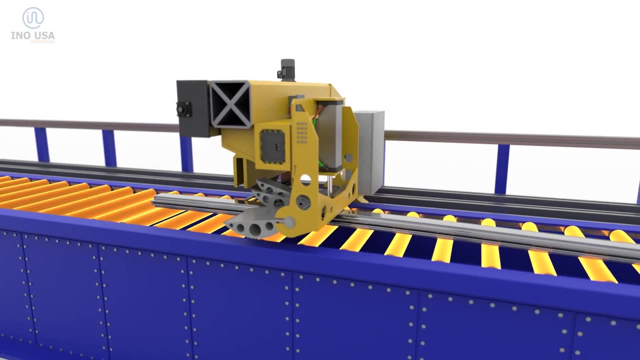 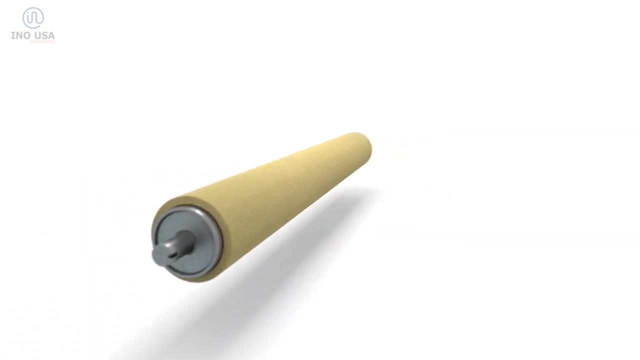 The run-out is a very long chain-driven roller system or an idler roller conveyor system that keeps moving the profile further down the line. The rollers are also covered with heat-resistant and non-marking felt covers. As the profile has cooled down a bit, the roller covers featured on the run-out table. 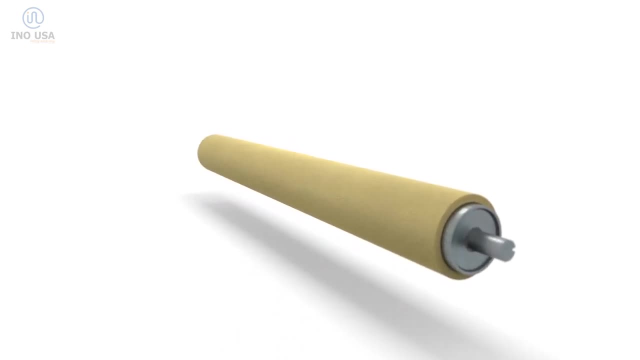 will be exposed to temperatures lower than on the lead-out table. These felt roller covers are normally made of 100% aramid fibers like Kevlar. Kevlar can withstand temperatures up to 900 degrees Fahrenheit for short periods of time. 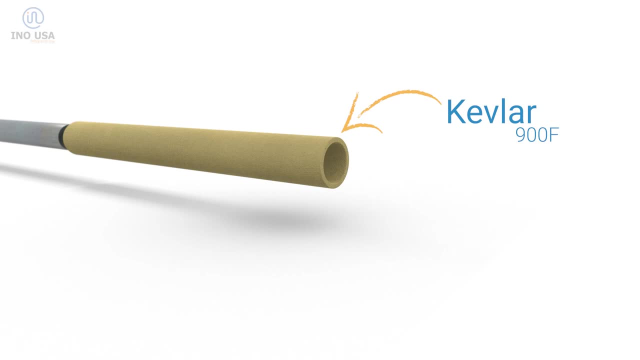 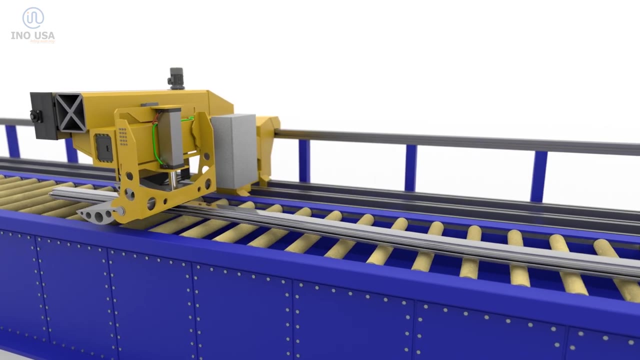 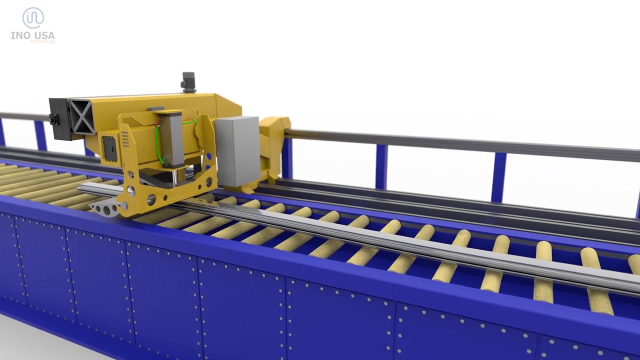 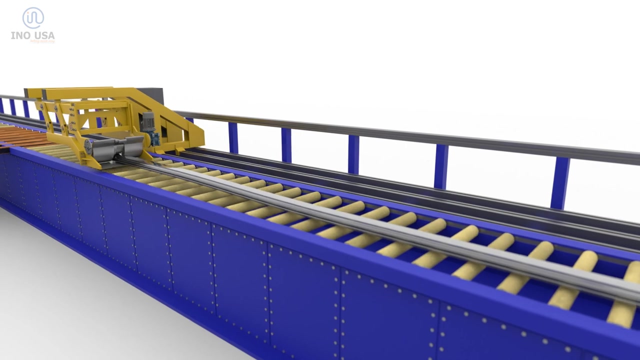 The felt can also be treated with resin as to make the roller cover harder and more resistant to abrasion, Depending on how long the extrusion is, sometimes it gets cut by a saw called the hot extrusion saw, Sometimes it is a separate machine and other times is built within the puller. 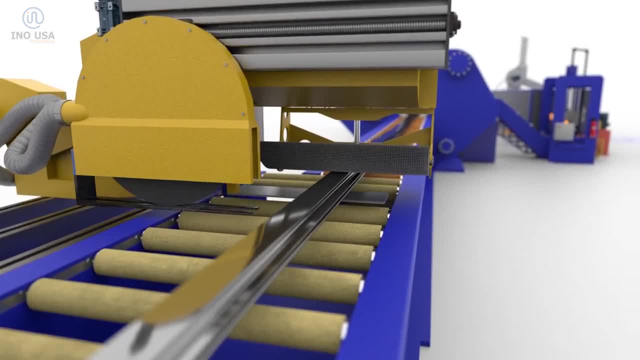 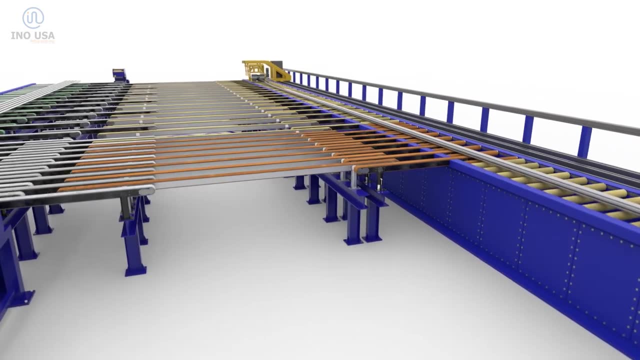 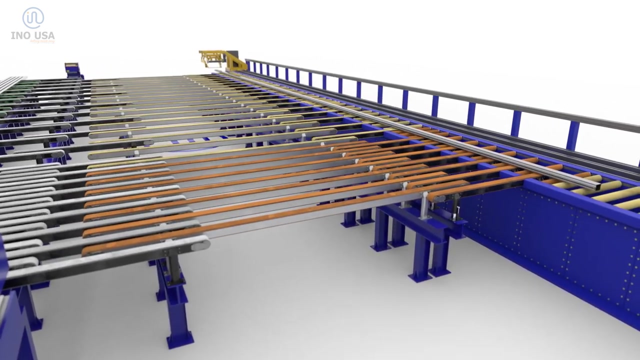 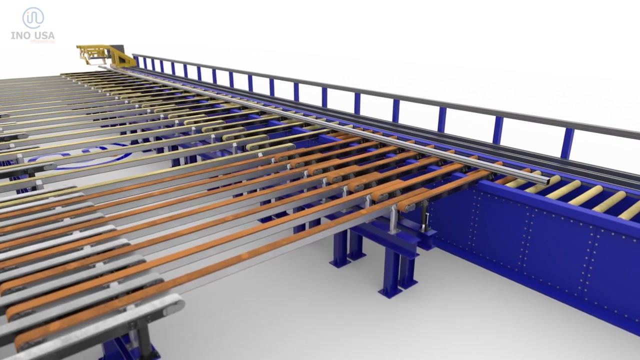 and it is called the flying hot extrusion saw. Between the rollers there are conveyor belts that line up the roll-out. These are the conveyor belts that are attached to the roller. They lift the profile and move it to the side. The transfers are normally done by felt belts, although some systems use a walking beam. 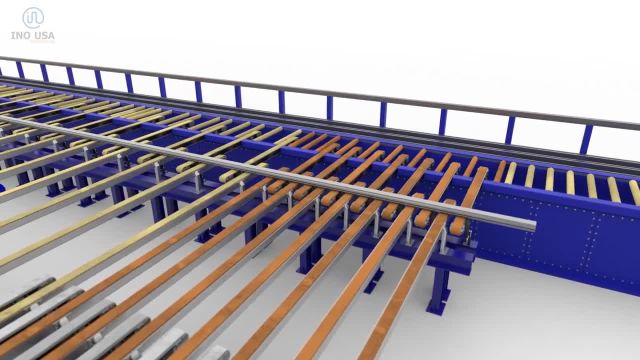 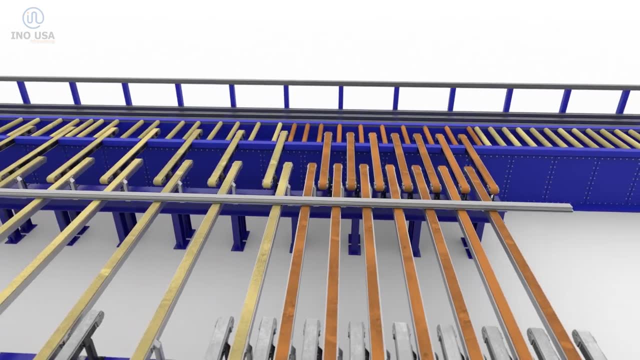 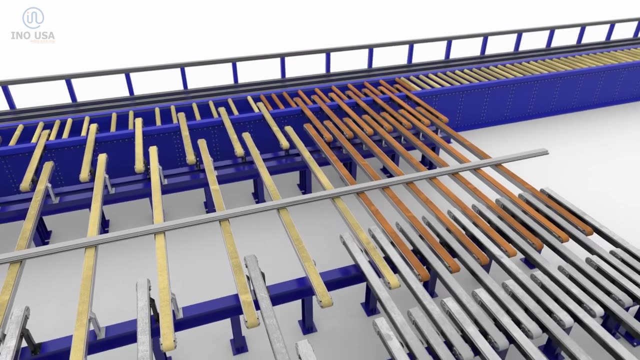 which is a beam that moves up and down with a forward motion as to walk the profile down the line. The profile moves to another set of belts called the first cooling table, where high-temperature resistant felt belts slowly move the profile down the line as it cools down. 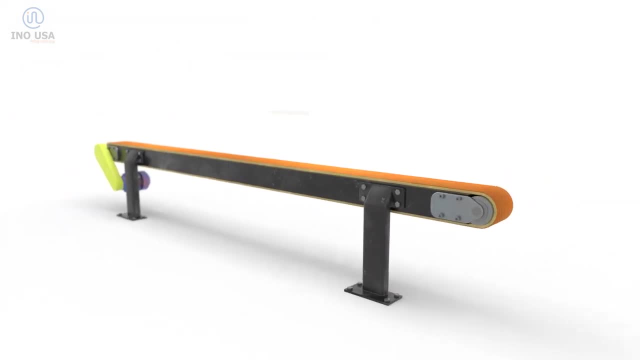 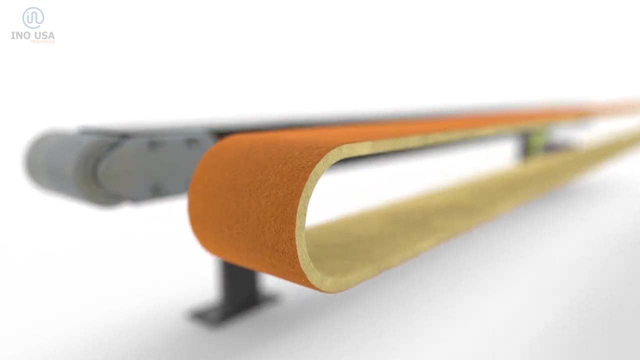 The first belts on both the lead-out table and the first cooling table are exposed to the tail end of the extrusion. The tail end of the extrusion still holds some high heat and these belts move slow Because of this. the best belt to use is a felt featuring our friend PBO on the top and aramid fiber like Kevlar on the bottom. 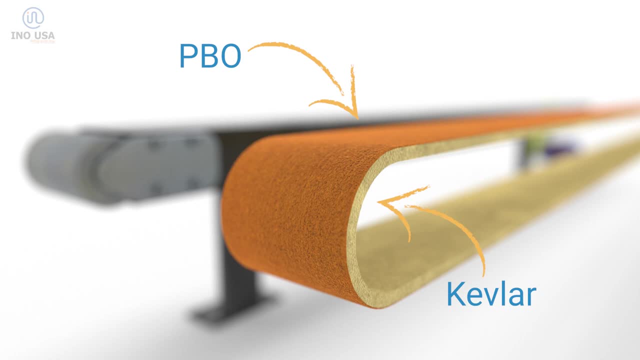 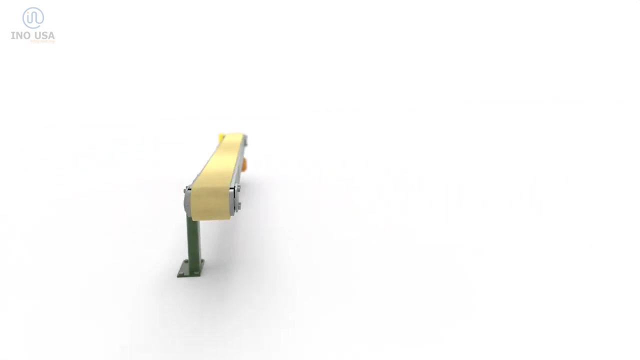 The belt has a scrim or woven textile reinforcement on the lower bottom to give the belt tensile strength to avoid stretching. These scrims are normally done out of polyester or aramid fiber. The rest of the lead-out table and first cooling table belts are exposed to lower temperatures. 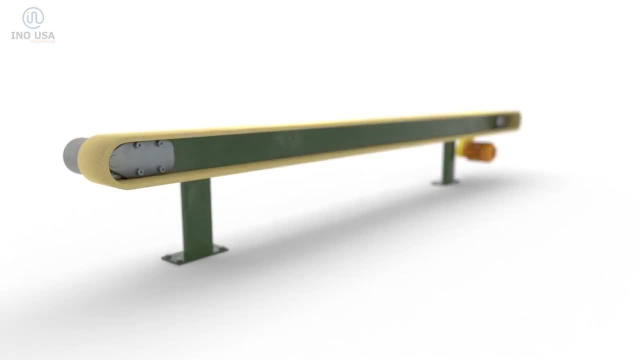 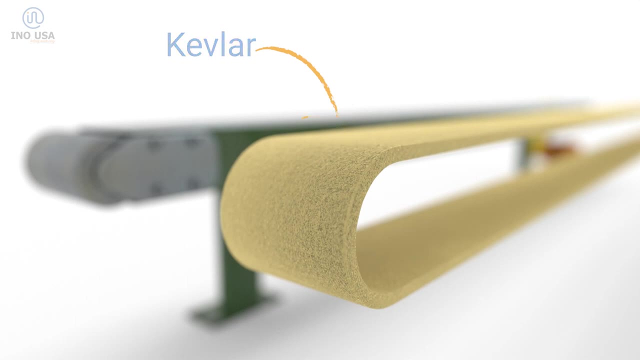 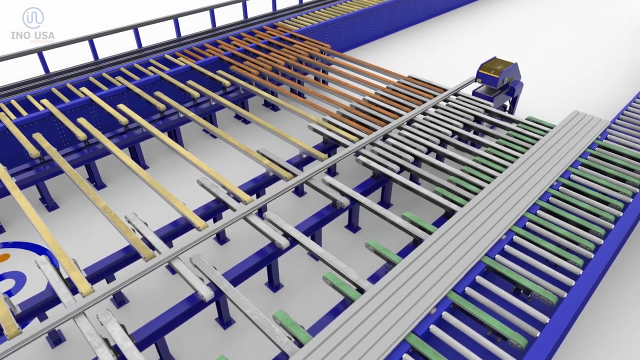 so normally belts made out of 100% aramid fiber, such as Kevlar, are used here. Just like the previous belts, these belts also have a scrim fabric reinforcement to avoid stretching. From the first cooling table, the profiles get transferred to a second cooling table for a stretching operation. 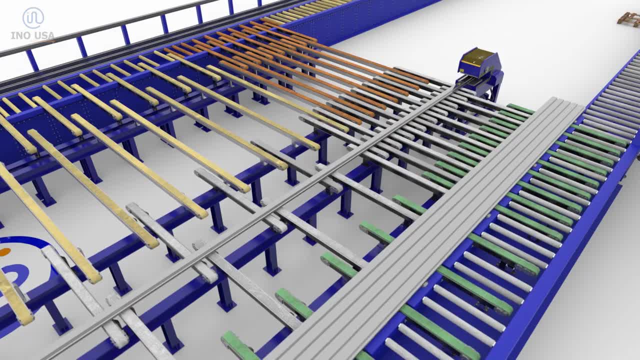 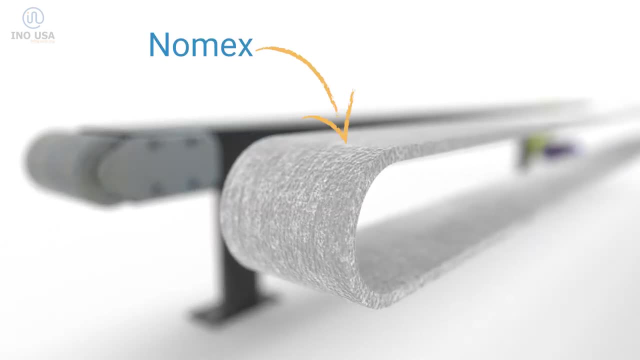 On this table, the profiles are transferred to a second cooling table for a stretching operation to intermittent temperatures up to 450°F. If the profile has cooled down faster, then other lower-cost synthetic fibers can be used, like polyester. Polyester can resist temperatures. 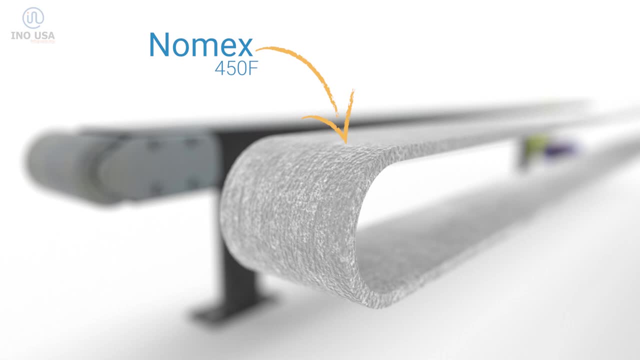 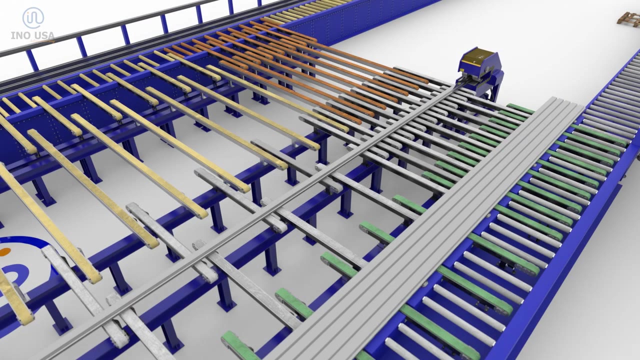 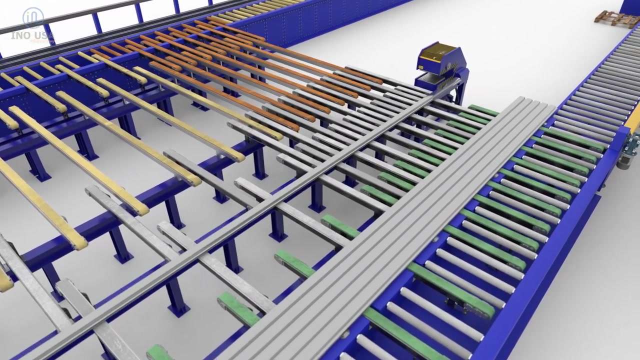 up to 300°F for short periods of time And, just like with the roller covers, these belts can be treated with resin to make them more abrasion-resistant. Two hydraulic clams pull the profile from opposite sides to stretch it and make sure it is straight. After the profile is stretched, it moves down the line to the storage tables. 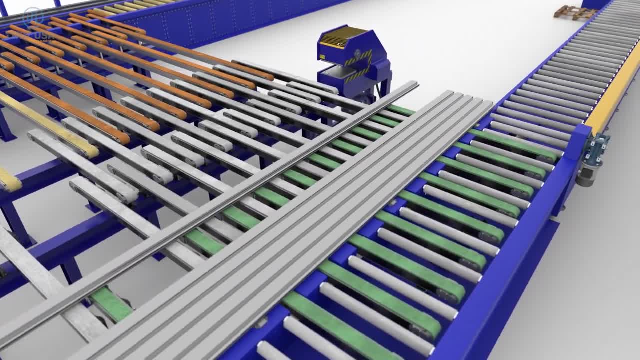 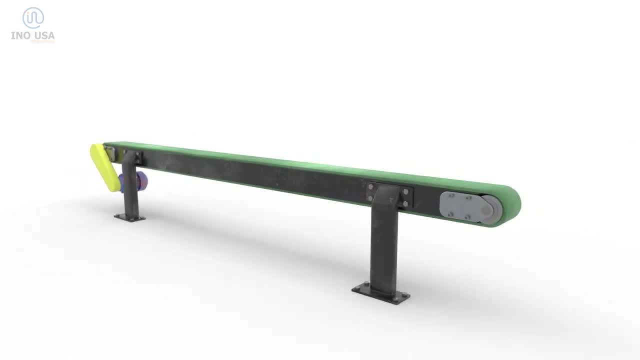 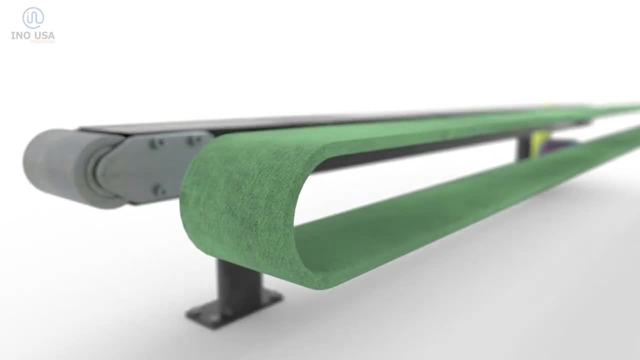 via felt belts or walking beams, Like on the second cooling table. the profile here is much cooler. The storage table belts aren't exposed to high heat, so polyester is the best fiber to use here, which is good for up to 300°F intermittent. The most common belts used in 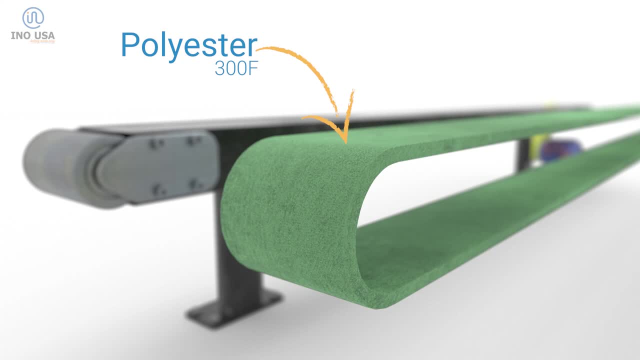 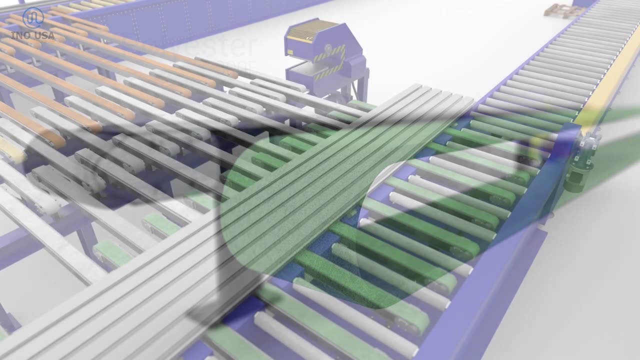 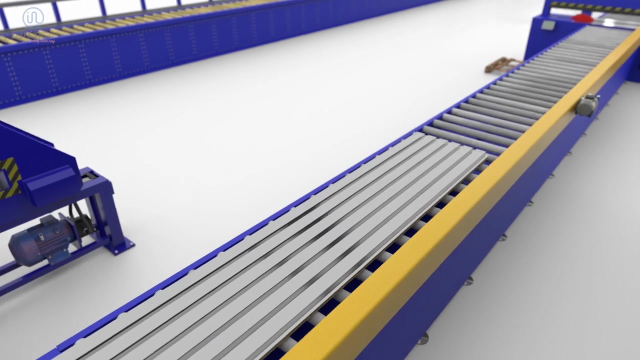 the industry are either green or black polyester impregnated with nitrile for more abrasion resistance Or the more economical regular white polyester felt. The storage table ends on another long roller bed. These rollers have polyester felt covers or plastic covers. The rollers, whether driven or gravity, move the profiles to the finish. 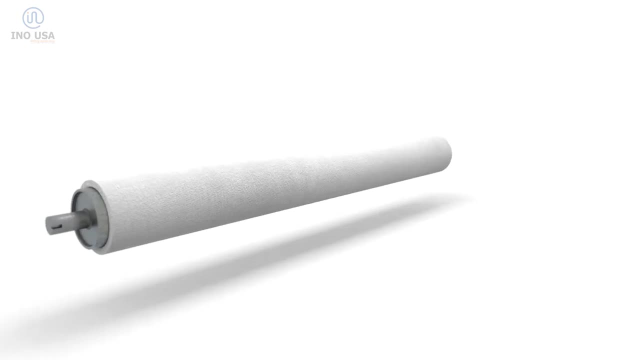 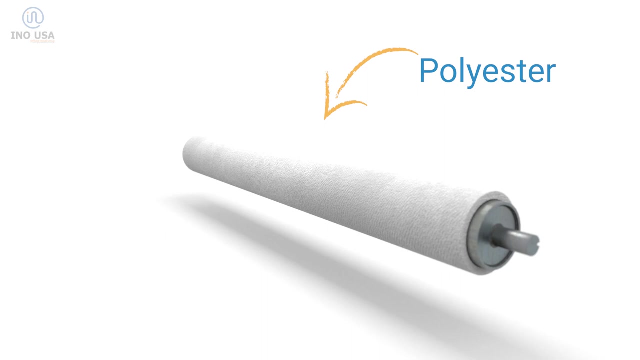 saw or the batch saw. The most cost-efficient solution for this roller bed is to use polyester felt roller covers. The temperature here is low, so polyester is the best fiber to be used, And because it is a fiber-free material, polyester is the best fiber to be used, And because it 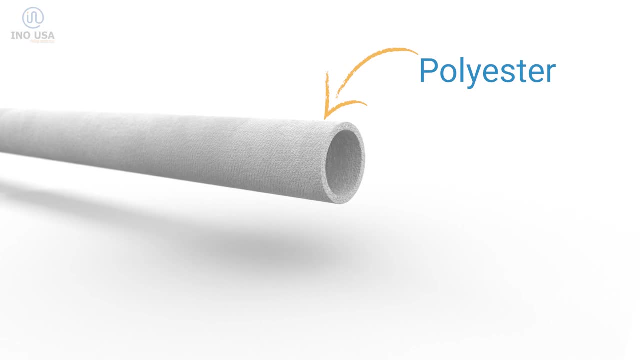 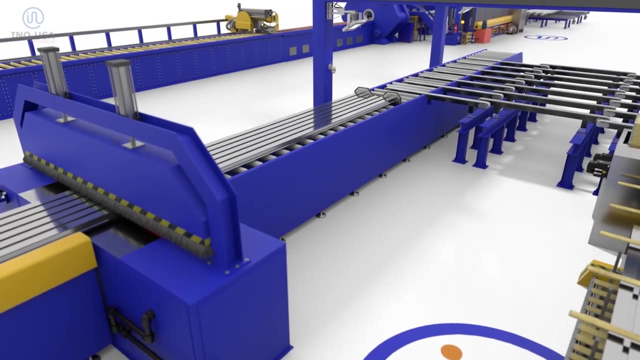 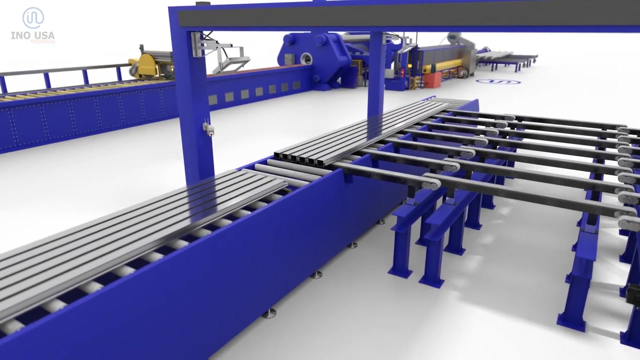 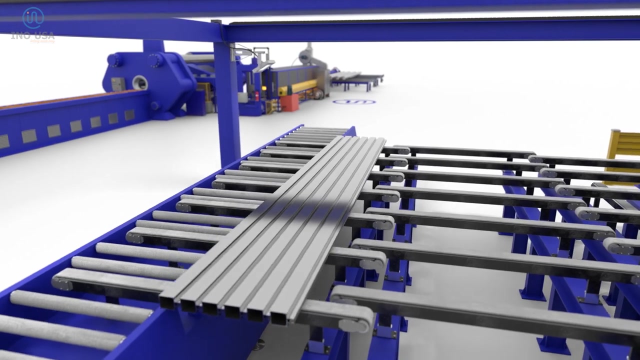 is a felt roller cover. the roller will be nice and easy on the profile and it won't scratch it or leave marks. The finish saw cuts the profiles to the exact length needed. A set of two or three tables of belts move the profile down to the stacker or cradle. 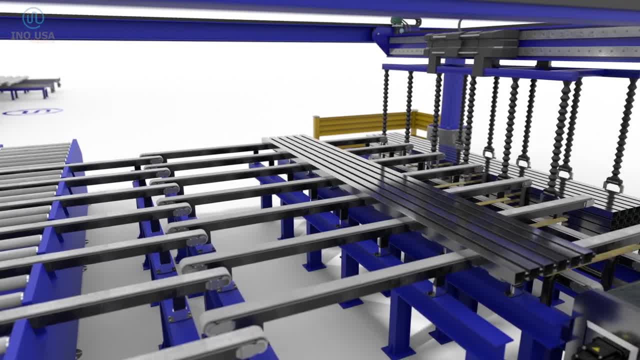 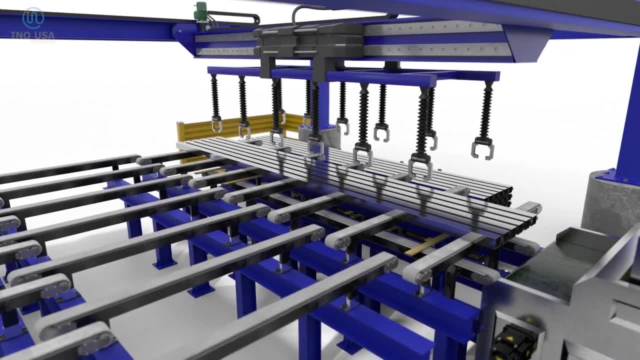 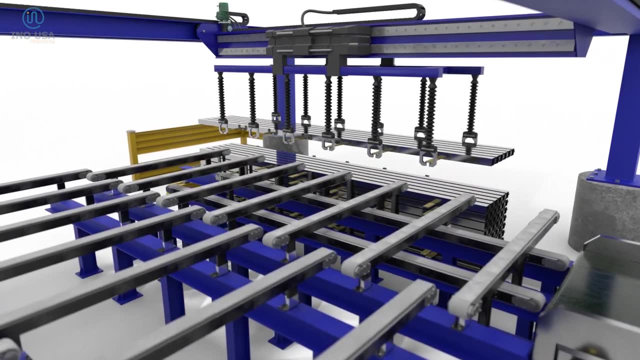 On the stacker. the profile sits on a separator bar fitted in the center of the profile. The rest are fitted inside a meta-aramid sleeve as to not scratch the felt felt product. Several layers of the aluminum profile get stacked with separator bars in between. 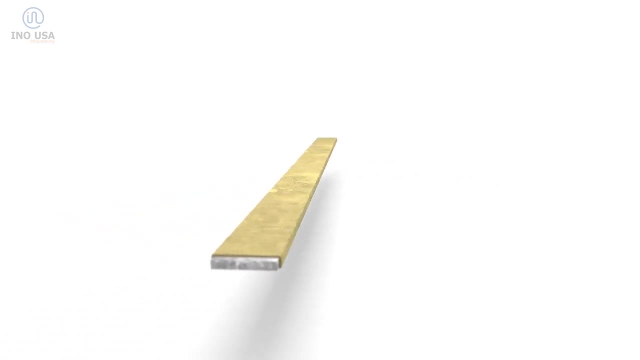 The separator bars are normally put inside a felt sleeve. These felt sleeves are there to avoid direct contact between the metal and the extrusion, as to not damage the extrusion. The most common fibers used here are the meta-aramid fibers, such as noses, 좋아s, gates and 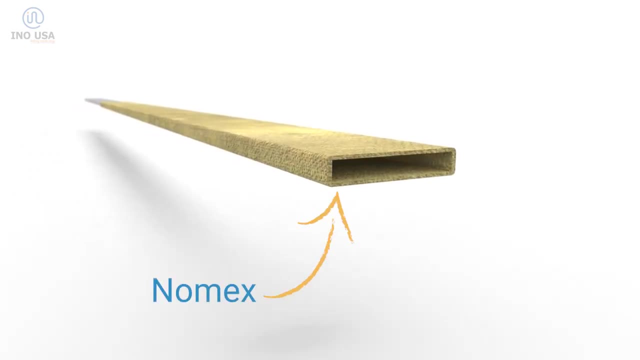 orroids: A wraps section with thelong goes-on square fabric on each side, The back side of the back section with the long goes-on square fabric, an outerPass and overall thickness as Nomex. These are the recommended fibers because the sleeve will be exposed to high 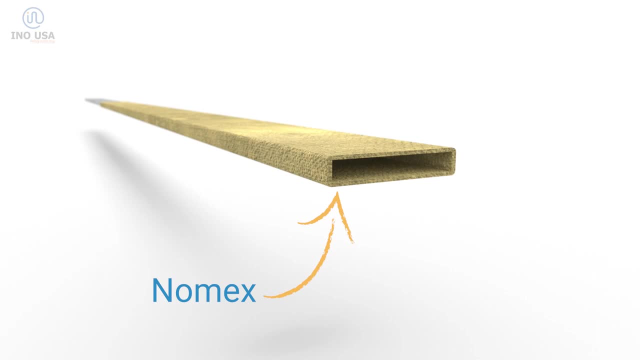 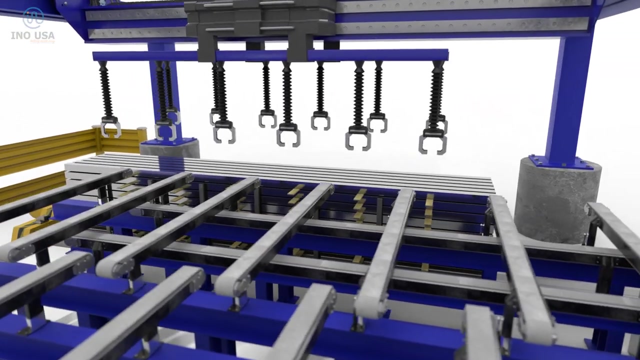 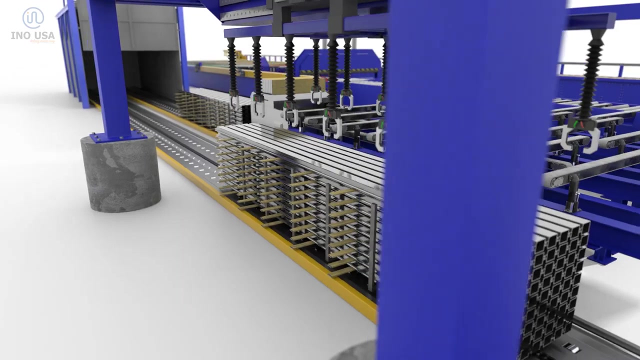 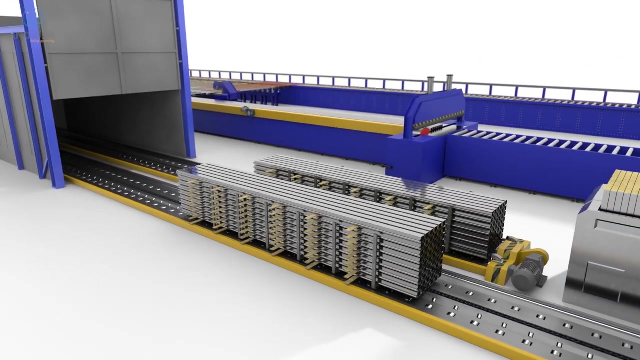 temperatures in the aging oven afterwards. The sleeves can be closed on one end and open on the other like a sock, or they can be open on both ends. They're normally quite thin, around 2mm thick or so. The stacked profiles get transferred to an aging oven. In the aging oven, the aluminum 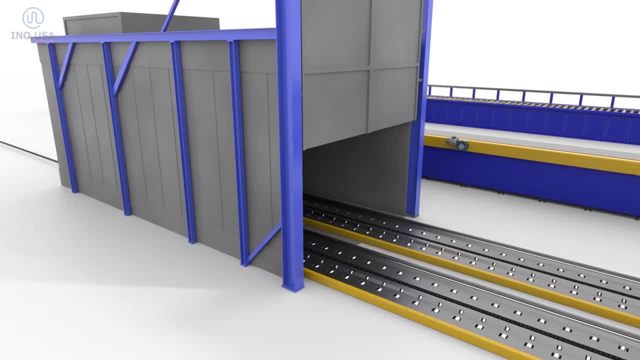 hardens at temperatures from 250 to 400 degrees. In some cases, profiles go through an annealing process at higher temperatures.